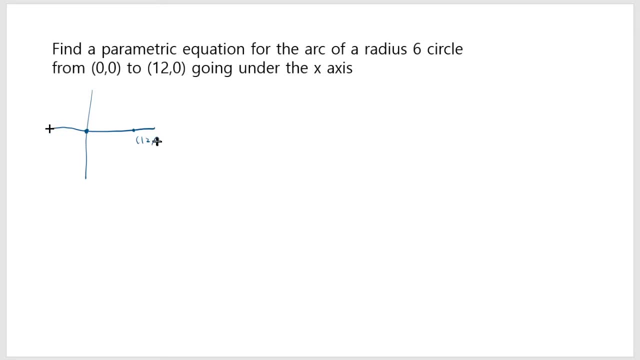 And it's radius 6th circle. so this is 0 to 12,, that's 12,. so this has to be the diameter, because if you have a circle, the longest distance between two points is the diameter, and the radius 6th circle has 12 as its diameter, right. 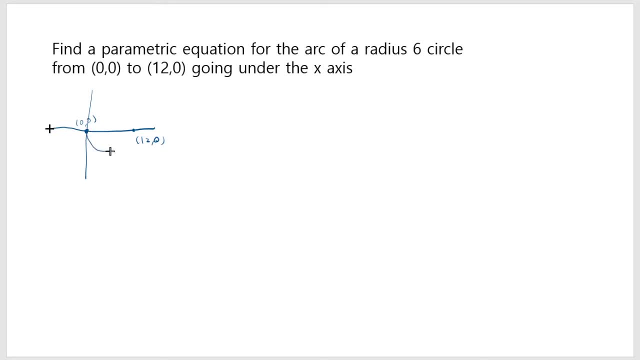 So it must be like. It's like the half circle and it's going under the x-axis, so this is what we want to represent. Okay, it's just half circle. So for this one, it's helpful to start from the usual radius. 6th circle. 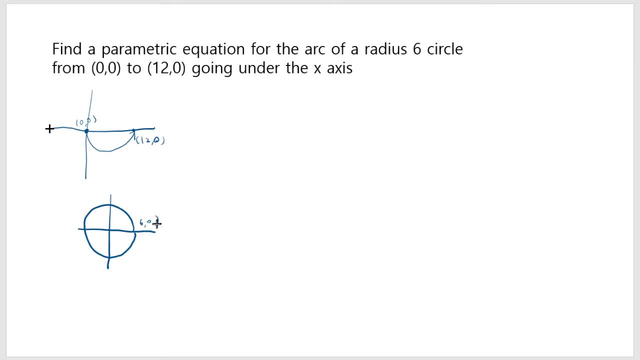 So let's say: this is and this is Okay. So let's say: this is this point right here. and we know that this circle is parametrized by 6 times cos, 6 times sin. okay, So if you set this equals to RT, then this gives you the parametrization of the circle. 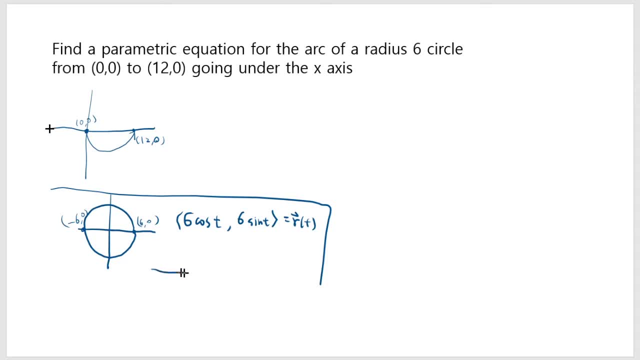 Now what's happened from here to there is? I think two things happened. It shifted 6 to the right, so that the circle is now not centered at the origin, but centered at 6, 0. And therefore, to move everything to the right by 6,, you need to make RT as 6 cos. 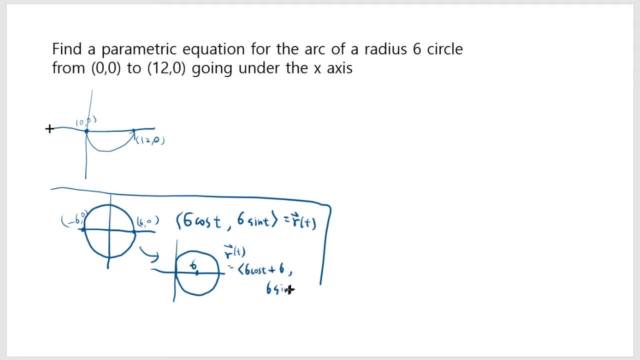 plus 6, 6 sin. Okay, So that's good. Okay, So now you can see that since the full story, you see, it's going this way, but it's not the full circle, It's the half circle. So remember, this would be when T is 0 and this would be when T is equal to pi, because 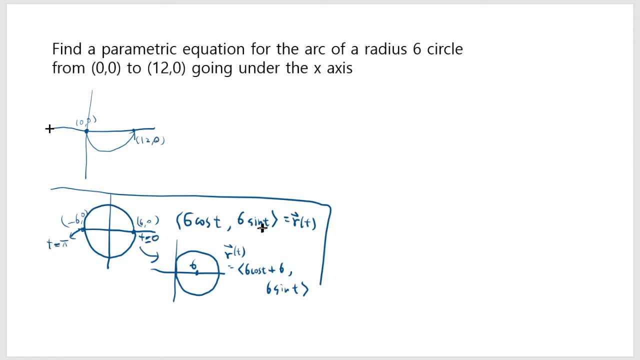 when T is pi, cos is negative 1 and sin is 0. so you do get 6, 0.. No, I'm sorry, negative 6, 0 when T is pi. So you, Okay, do have negative 6 comma 0 when t is pi and then when t is after pi, it for. 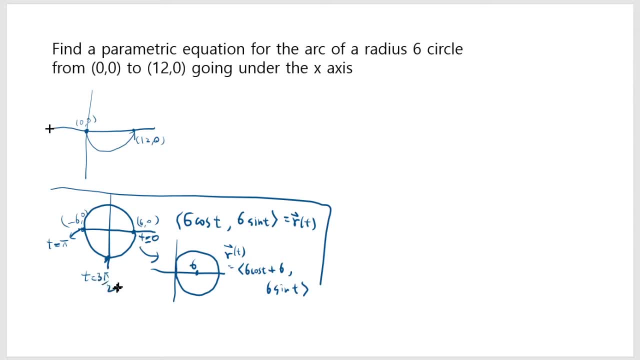 example right here would be when t is equal to 3, pi over 2, and then arrives at here. so it's really, it really starts here and then finishes here. okay, so it's really this part that we want and to to denote that it's really this part we 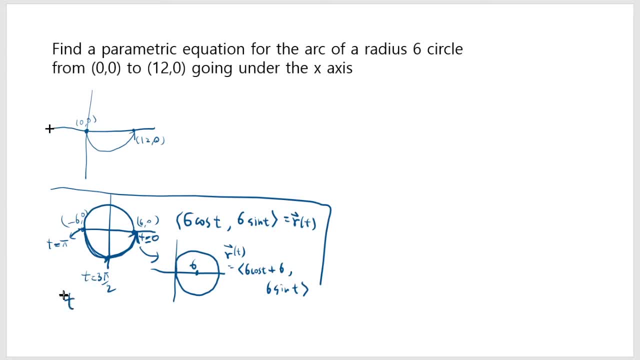 want. we should say t is between pi until 2 pi, because if it's 2 pi you come back to here. right, and this applies in the same way to this one, if you just want the bottom circle. so the answer to this would be that RT should be 6 cosine t. 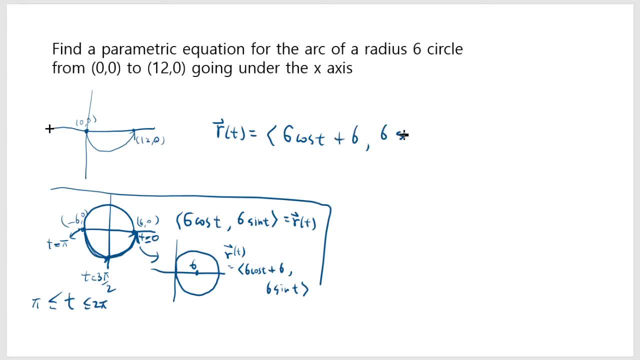 plus 6, 6 sine t with t between pi to 2 pi. now note that this is not the only answer. it's a parametric equation. it's not the only answer. if you're curious to know what other answers there are, for example, you can rewrite t as 2t, 2t and make t go. 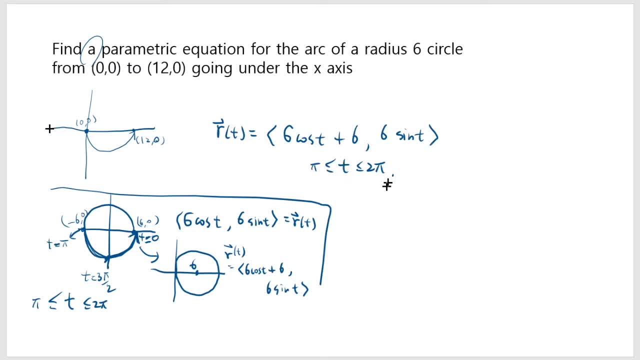 from pi over 2 to pi. that's. that's a legit answer. that will give you the exact same beginning and end points, and the difference would be that it's going to travel through this double time. it'll be twice as fast. so that's another possible answer. another thing you can do is 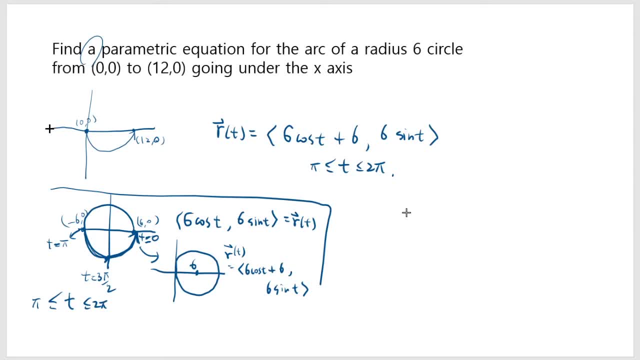 rather than using cosine and sine, you can also use sine and cosine, so alternatively out answer: there are infinitely many because you can change the speed. okay, but L tensor- I want to mention the one that uses sine- would be 6 sine of t plus 6 and 6 cosine of t, and what happens is: 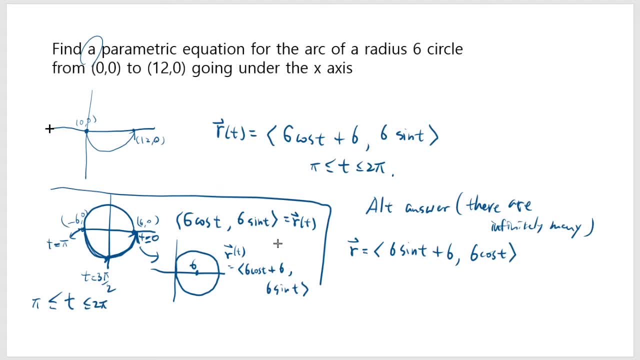 that sine pi over 2, sine pi over 2, sine pi over 2- sorry, sorry, cosine, pi over 2 to 3, pi over 2 makes this negative. so we know that that's negative and from if you look at the sine graph, sine graph is like that. so 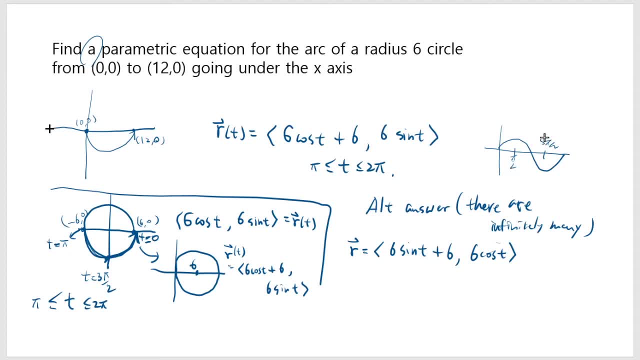 from pi over 2 to 3 pi over 2. the sine graph goes: it decreases, right, it goes from positive 1 to negative 1. okay, so i would require this to be a negative. okay, so, if you, if you have this, it just requires some trial and error and but. 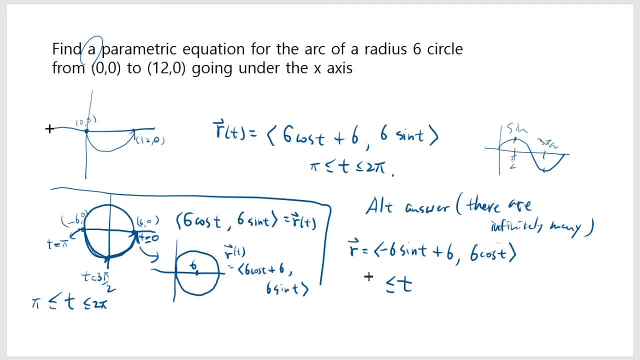 you can see that if you have this one with pi t being between pi over 2 to 3 pi over 2, then again it's going to give you the exact same trajectory. you can check this. but it's okay if you didn't understand. this is your reward. relation with cosine of t, which will be happy to use, is exactly also, but it's ok if you didn't. 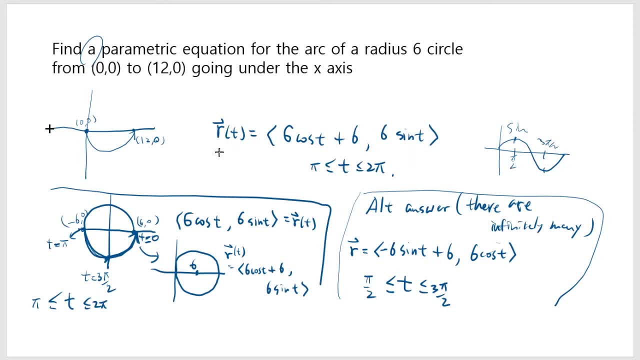 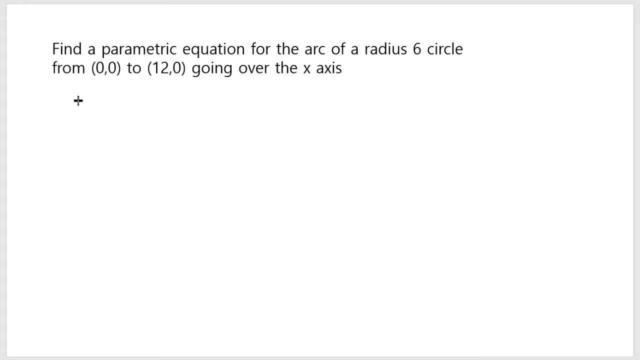 understand this. it's really this one you should be able to do. Now. this question is going under the x-axis, so let me show you how the answer would be different if it said it's going over the x-axis. If it's going over the x-axis, then it's the same picture, but instead you're going. 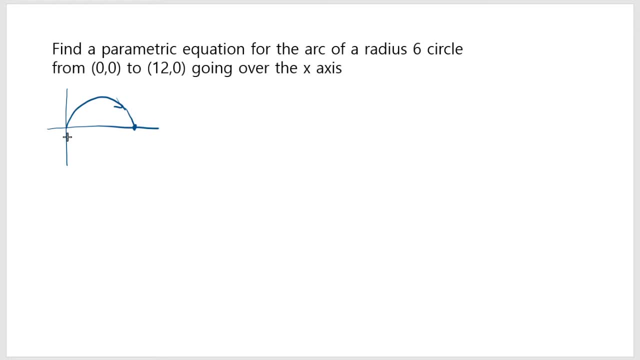 that way. Okay, so it's from 0 until 12,. you're going this way. So how does that work? Well, we can still use the same thing, but we have to start modifying the answer. So we know that it should be 6 cosine t, 6 sine t, because the radius is 6,. 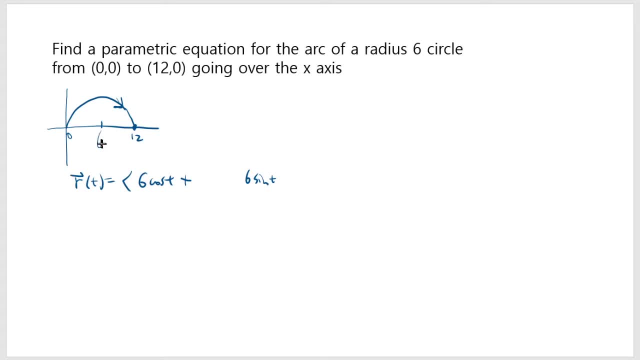 and then, since it's moved 6 to the right, the center of this circle is no longer 0, 0. It's 6 moved to the right, so I add 6 to here. Now, if the circle went up then I would have added 6 to here. 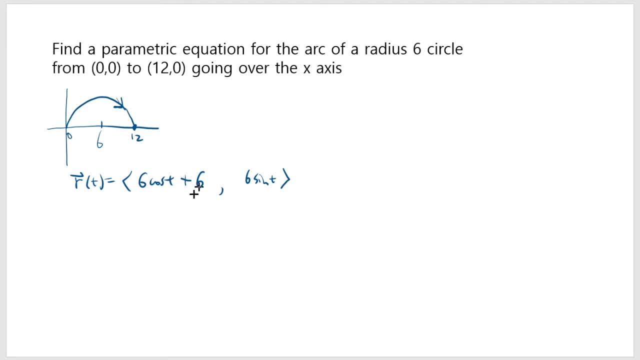 instead. okay, So you should be able to figure out what to add just by looking at the change of the center, And then you have to think about what to add to the center. So you have to think about what to add to the center. So you have to think about what to add to the center, And then you have to think about 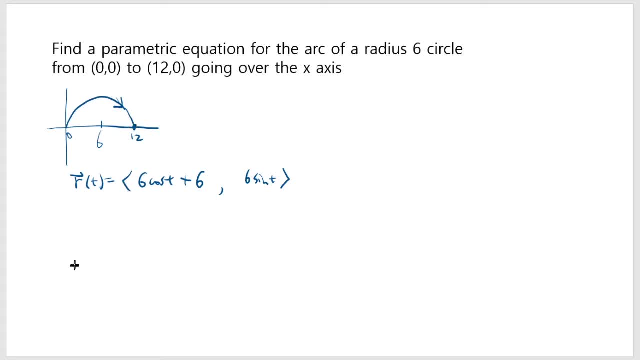 what would this be parameterized as? So in this circle, regular circle, this is t equal to 0, and this is t equals to pi. So if you go this way, then you're going to get t equal to 0 to t equals to pi. So you: 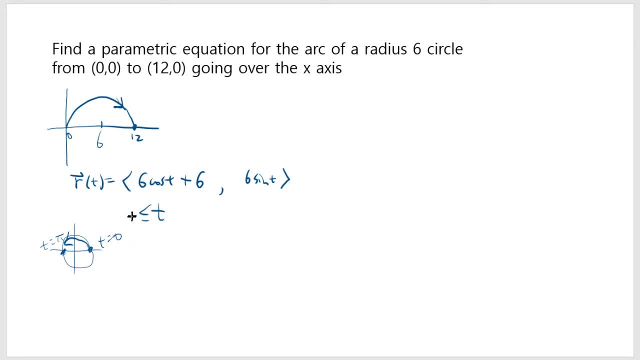 if you do t from 0 to pi, this is almost the answer, but this is so. this one, this one will give you the circle that's going this way, which is the opposite of what you want. okay, So how do you change this? Well, see, you want to start from. 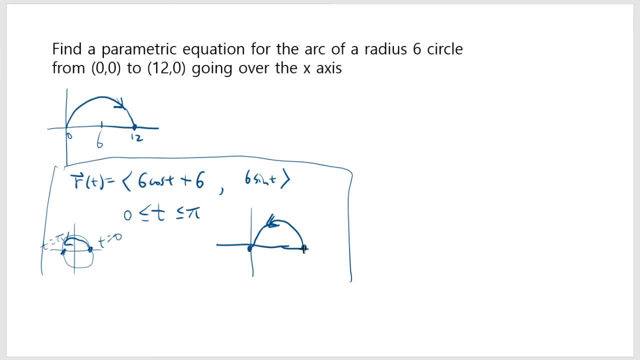 pi and you want to end at 0, right. So one nice thing you can do is replace t by pi minus t. If you replace t by pi minus t, then when t is 0, pi will be plugged in, so it will have the effect of starting from here, And when t is pi, you end up with this. So if you say rt equals to 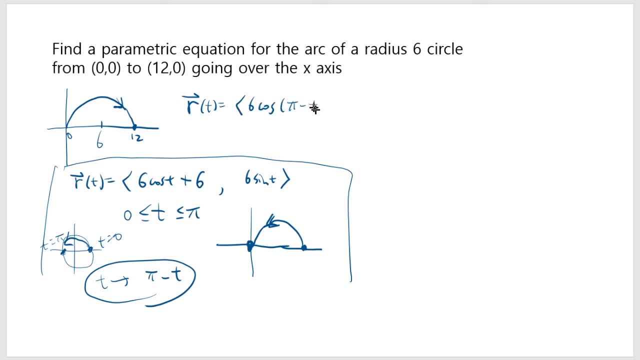 6 cosine pi minus t plus 6, 6 sine pi minus t, then this one will give you exactly what you want. okay, It starts from here and ends there, okay. And then you want to simplify these and you know- I mean I'm not so sure if you're doing some problems on WebWorks or some other platform- they might want, they might not want these pi minus t there. so you have to know how to simplify them, And to do that there are many ways, but I guess the more straightforward way is to use this sine sum formula, which is sine of a.